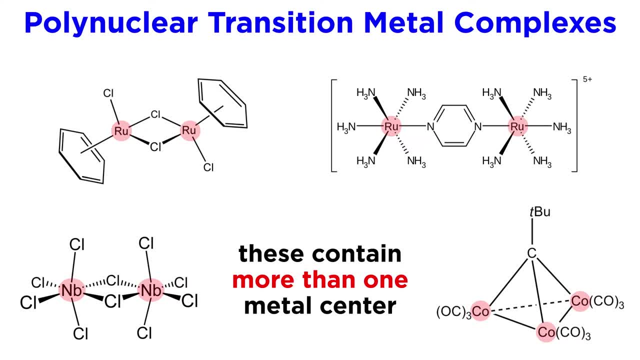 metal complexes. These are complexes involving more than one central metal atom, which we will frequently encounter. Each metal will be coordinated to some number of ligands, and then the metals will also usually have one or more bonds between them. As we mentioned in an earlier tutorial, this can be complicated by the presence of bridging ligands. These 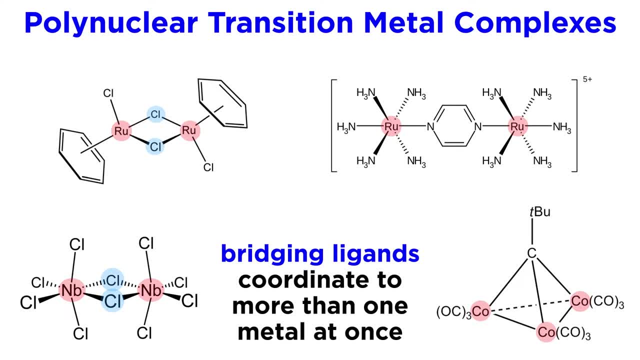 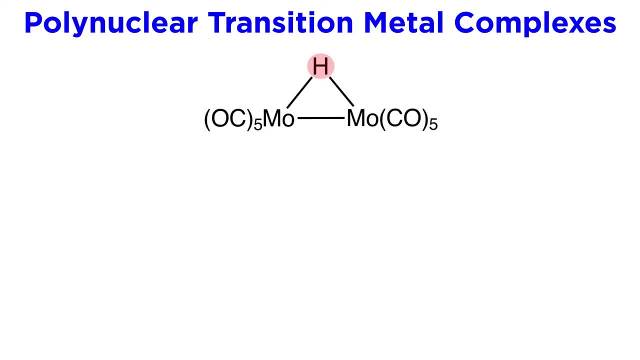 are ligands that are coordinated to more than one metal center at the same time, a feature that is expressed by the symbol mu preceding the ligand in the chemical formula. As we may recall, one counter-intuitive aspect of ligands is that they are not connected to. 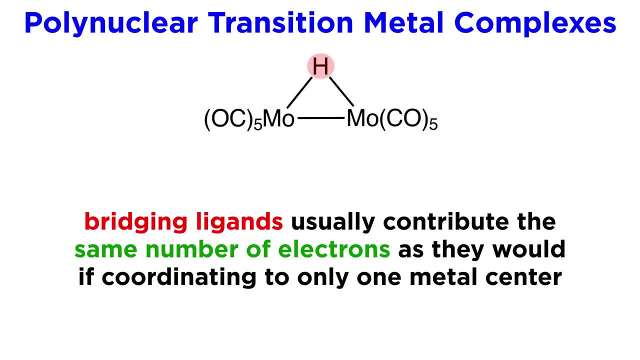 bridging ligands is that these ligands will usually contribute the same number of electrons to the complex as they would, if coordinated, to a single metal atom, even though we will depict two bonds instead of one, So a bridging hydrogen will still contribute only two electrons. 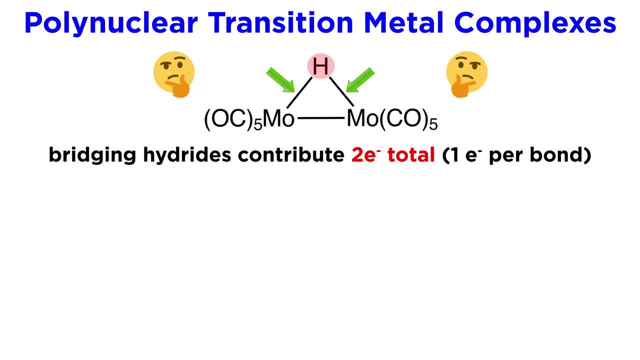 as we would expect from hydride. While it may seem absurd to see two bonds coming from a hydrogen atom, those two bonds actually contribute a total of only two electrons, which are distributed among two metal centers. Another exception is ligands with two or more lone pairs, like chlorine, which can 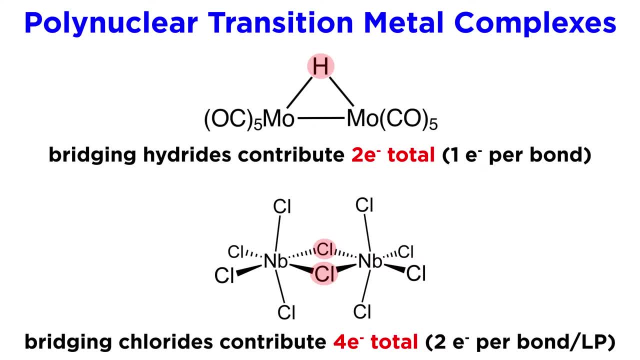 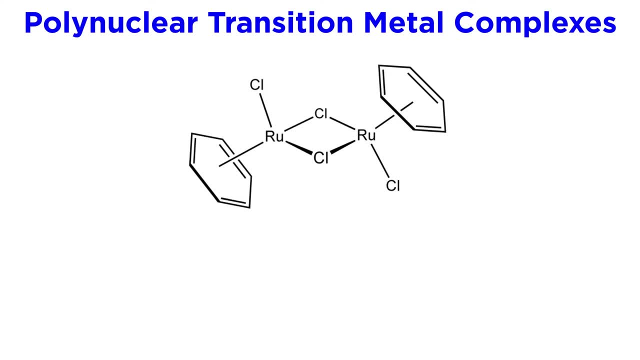 actually donate one lone pair to each metal, thereby contributing four electrons instead of the typical two. It is often the case that each metal center in such a complex is bound to the same set of ligands. Therefore, it can be easy to check whether the 18-electron rule is being satisfied. 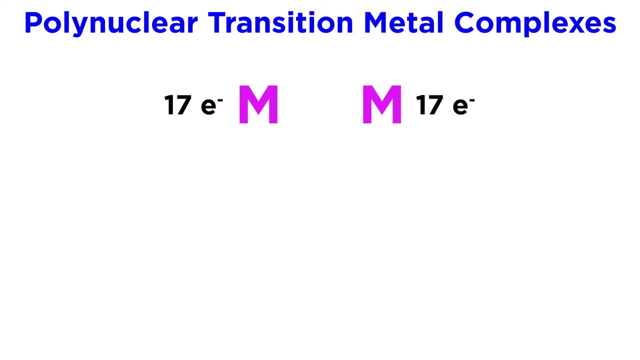 for each metal center. A common situation is that each metal will have an electron count of 17,, and then, to get to 18-electrons, it will have an electron count of 17,, and then, to get to 18,. they will each contribute one electron to a covalent bond between them. 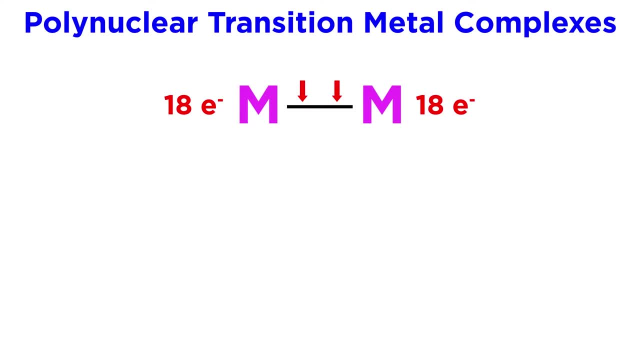 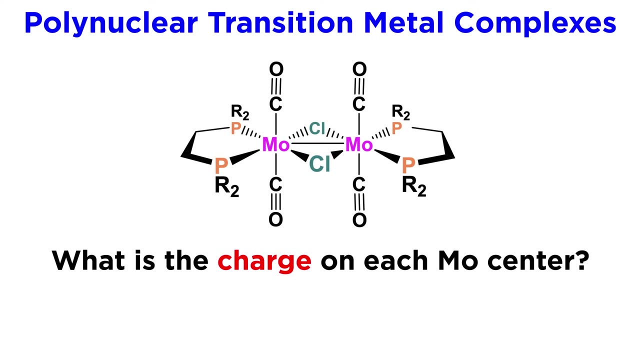 and this bond may be strong or weak depending on a variety of factors. Here is one such situation. We have two molybdenum centers, each of which is coordinated to two carbonyls: one bidentate diphosphine ligand and two bridging chlorines. When determining the charge, 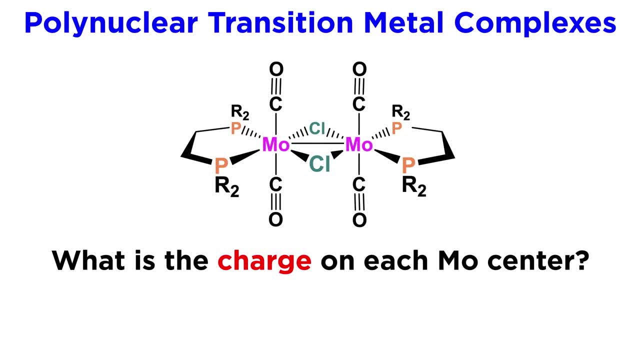 on the metal centers. we must be careful. apart from the neutral ligands, the bridging chlorines have a negative charge. When we determine the charge on the neutral ligands, the bridging chlorines have a negative charge. when we determine the charge on the neutral ligands, the bridging chlorines have a negative charge. 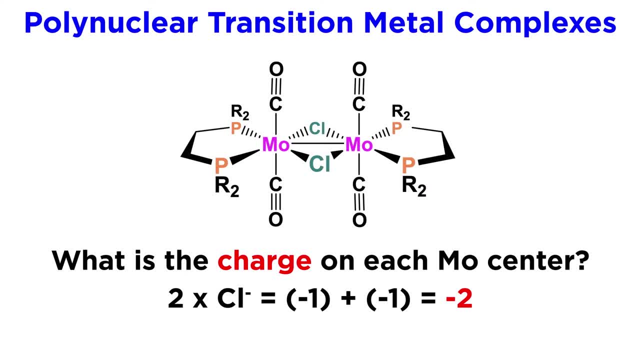 just as we would expect when coordinated to only one metal, but the two negative charges are distributed amongst two metal centers. This means that each metal must have a plus one charge to balance things out and get to neutral charge overall. Molybdenum is 5s1. 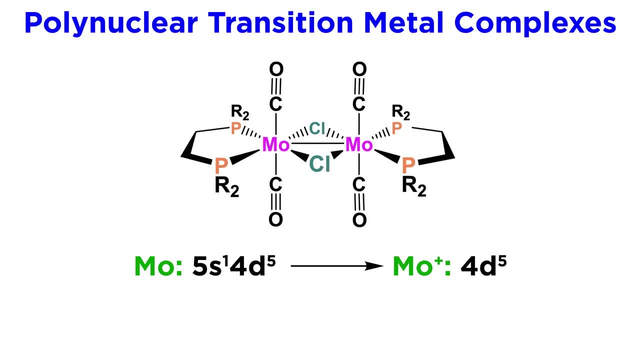 4d5, so the plus one cation will be 4d5, thereby contributing 5 electrons to the count. The bidentate phosphine contributes 4 electrons, 2 per phosphorous. the carbonyls contribute 2 electrons each, as do the bridging chlorines. 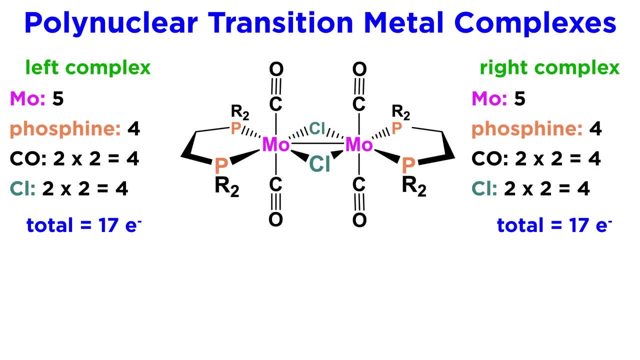 as they each contribute 2 electrons to each metal, That adds up to 17 electrons for each molybdenum center. so we simply add one covalent bond between the two metals to bump the total up to 18.. Now that we understand how this works, let's 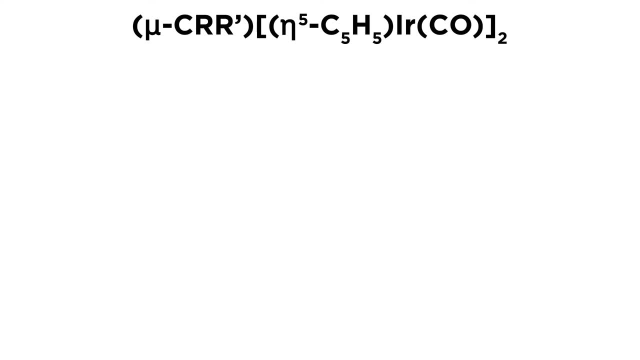 look at a few chemical formulae for polynuclear complexes and see if we can predict the structure, presuming that the metals are coordinatively saturated. This first one has a bridging alkylidene ligand and then we see an iridium center bound to a CP ligand and a carbonyl. and because 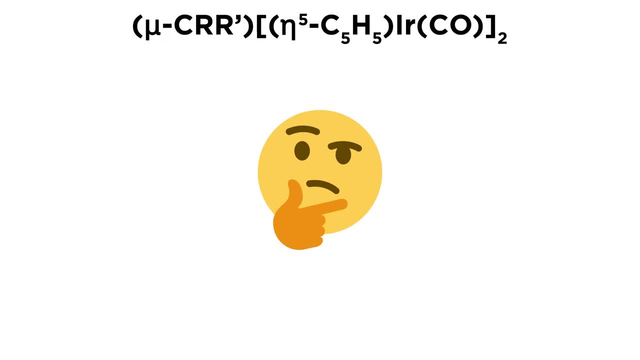 of the brackets. here we see that there are two of these. With this information, we can start to put together the structure, since we have two iridium atoms, each with the two ligands, and we can also put the bridging ligand. We simply have to figure out how many. 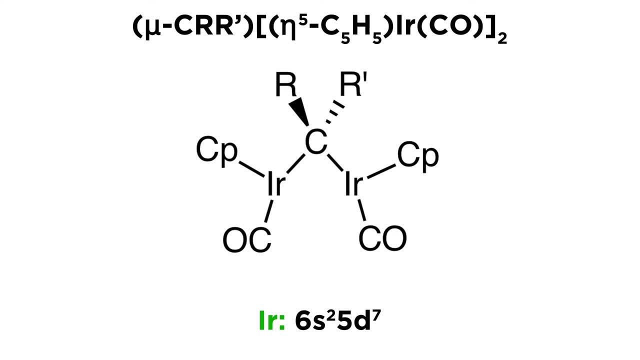 bonds are between them. So let's look at the structure. We have two iridium atoms, each with the two ligands, and we can also put the bridging ligand. We simply have to figure out how many bonds are between the metals. Now, iridium is 6s2, 5d7, so it has 9 valence electrons. The carbonyl is neutral. 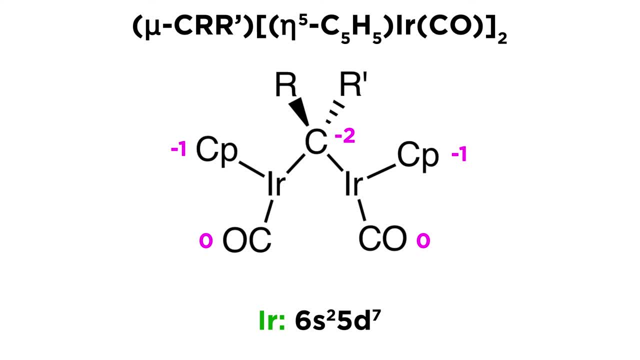 the CP ligand has a minus one charge and the alkylidene ligand has a minus two charge, which is distributed amongst the two metals because it is a bridging ligand. so we can think of it as minus one going to each metal. That's a total of minus two to each metal. 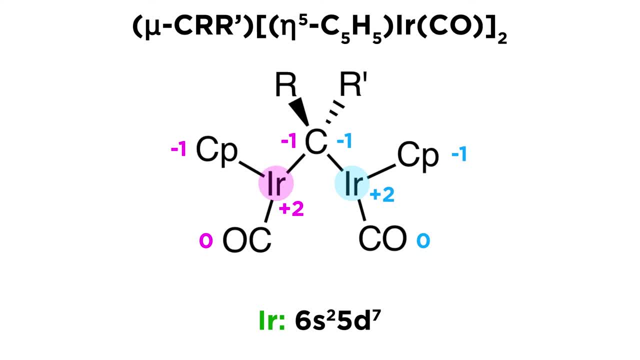 so they must each be in the plus two oxidation state, since the complex is neutral, overall 9 valence electrons minus two is seven, The seven from the metal plus six from the CP ligand, plus two from the carbonyl, plus two from alkylidene. since 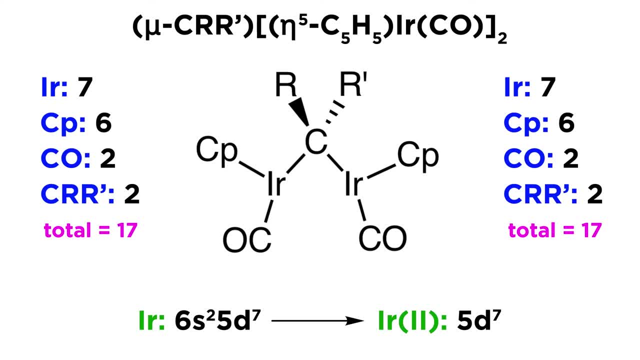 its four electrons are split up between two metals, gives us a total of 17 electrons surrounding each iridium center. Therefore, we simply add one bond between the metals, and that will bring us to 18 for both of them, and we end up with this structure resembling a 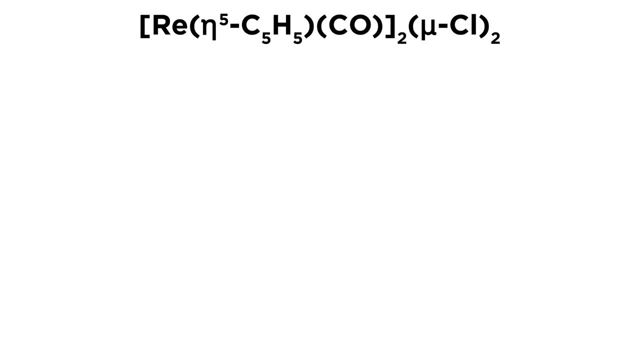 three-membered ring. Let's try one more. We have a binuclear rhenium complex, where each metal is bound to a CP ligand and a carbonyl, and then there are two bridging chlorines. Rhenium is 6s2- 5d5,. 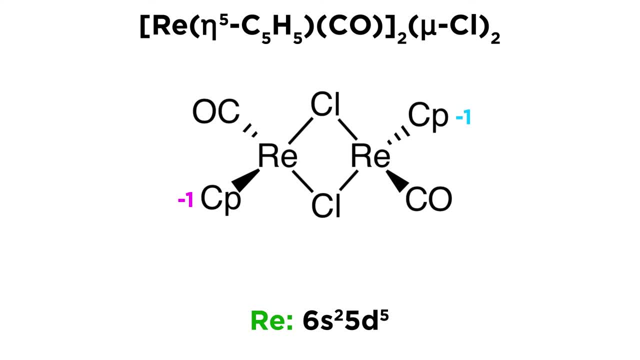 so the metals have seven valence electrons, The CP ligand is minus one and the chlorines are each minus one, but coordinated to two metals. so that's minus one to each metal, Plus two. each rhenium center must be in the plus two oxidation state, so we drop the S. 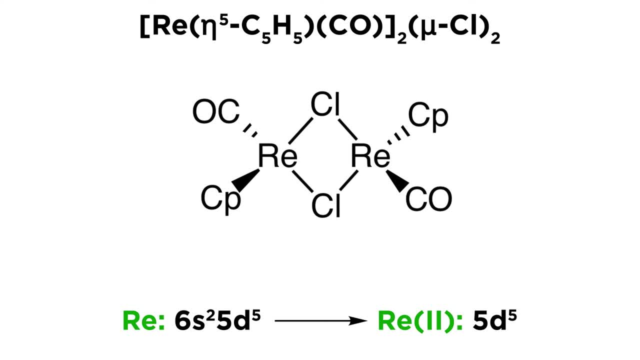 electrons to give five valence electrons, Five plus the six from the CP, plus two from the carbonyl, plus two from each bridging chlorine, or four total gives us a total of 17 electrons To get to 18, we will simply draw one bond between the metals and that's. 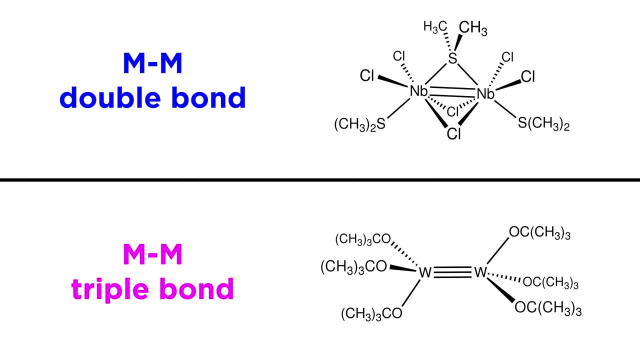 our complex. Other complexes may have two or even three bonds between the metal atoms. so we have to draw one bond between the metals, and that's our complex. So we have to draw one bond between the metals, and that's our complex. 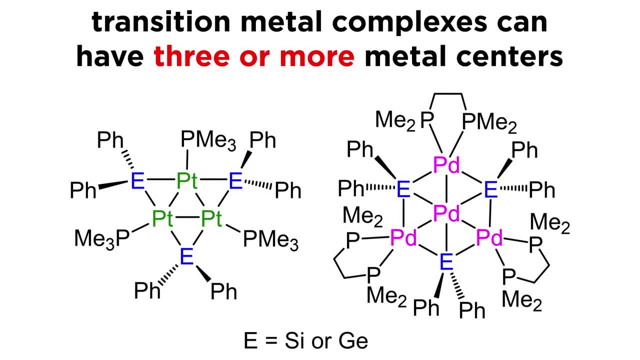 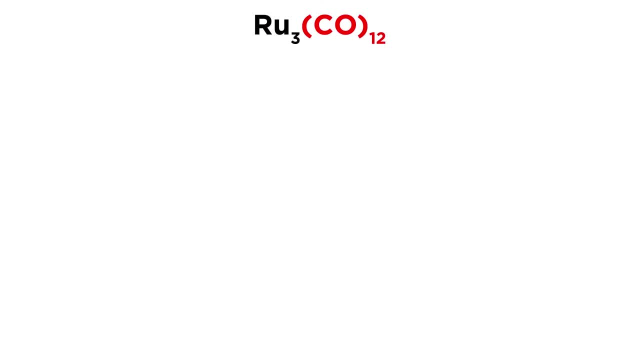 And of course there are complexes with more than two metal atoms. Just to see one example, this complex has three ruthenium atoms and twelve carbonyl ligands. How can we make this work? Presuming symmetry, each ruthenium should have four carbonyls. None of the ligands. 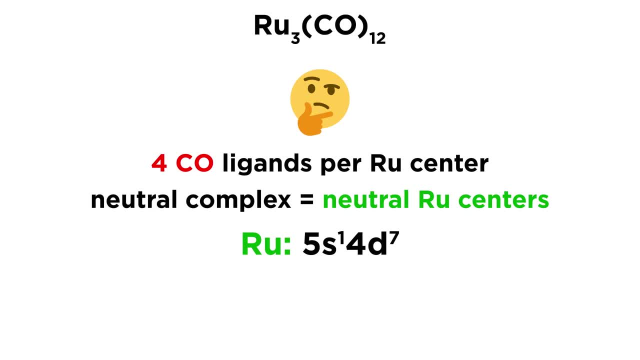 have any charge. so the metals are neutral, which means they have all eight valence electrons, Plus eight from the four carbonyls gets us to 16, so each metal needs two more electrons. This can happen if each metal is bound to the other two, so we can set up a three-membered. 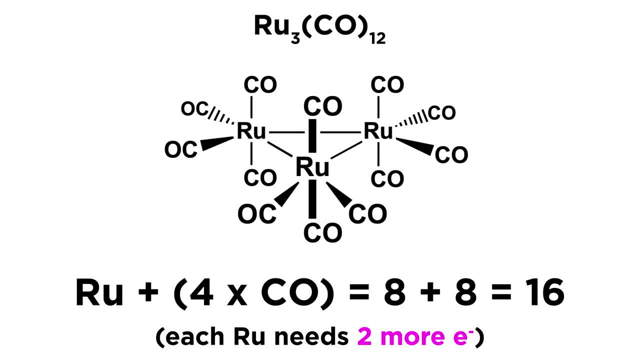 ring like this and the ligands occupy the other octahedral sites. It is also possible to arrive at a viable structure without any metal-metal bonds and using bridging ligands. However, the structure shown here can be confirmed by spectroscopy. We may see interesting substances.